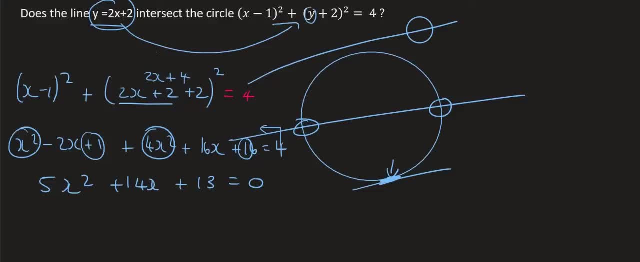 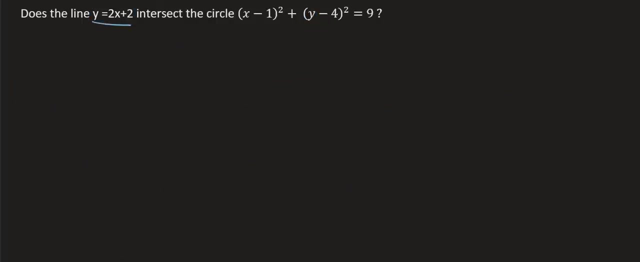 quadratic formula. for this you should get an x value of nope. we don't get an x answer, we get an error on the calculator. What that means is that that line does not cut the circle, so it looks like that. Here's another one. so we're going to take the same line and we're 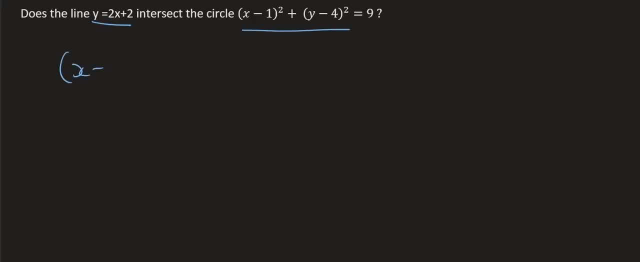 going to see if it intersects this circle. So, once again, all we need to do is plug the straight line equation into the place of y. so that's going to give us 2x plus 2 minus 4.. You see, so that 2x. 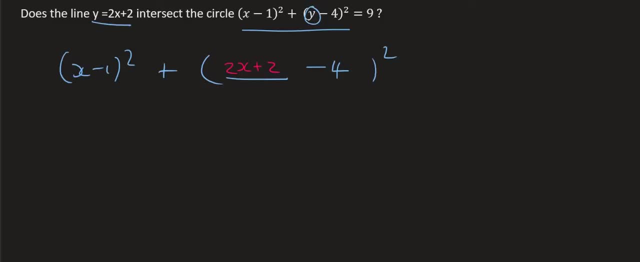 plus 2 is from the straight line. So I replace that y with the straight line's y, and then I say equals to 9.. I can then go multiply out This plus 2 and this minus 4, that's just going to give us minus 2, and so if I had to, 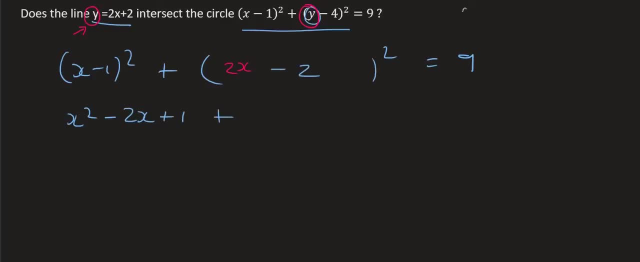 multiply that out. you can do this the long way, where you put the two brackets next to each other like this, but I'm just doing it the quick way. So that's going to give us 4x squared minus 8x plus 4 equals to 9.. I'm then going to put all the x squareds together, so that's going to give 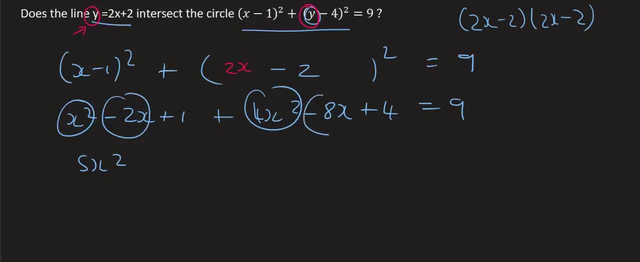 us 5x squared, The x's will go together, so that's going to give us minus 10, and then, if you put all the numbers together, that's going to give us 5 minus 9, which is minus 4.. We then use the quadratic. 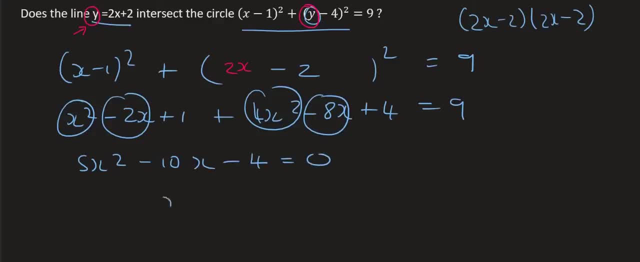 formula, and once you've done the quadratic formula, you should get answers of 2.34 and negative 0.34.. So does the line cut the circle? Yes, and because we've got two answers, it means that we've got the right answer. So we're going to put all the x's together and then 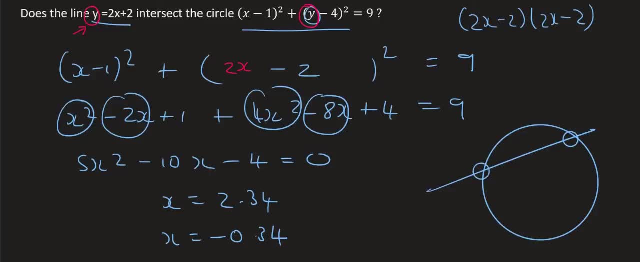 it cuts it in two different places, and so we would call that line a secant. Okay, let me write that out for you. A secant cuts the line in two places. If we only got one answer, such as x equals to 1 and x equals to 1, so they're the same value, then it would be a tangent. 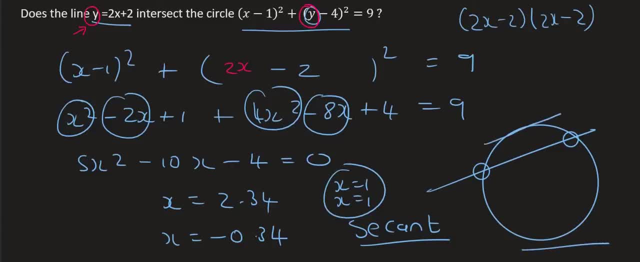 and if we got an error then it means it doesn't cut the line at all. Then if you wanted to find the y values to those points, you would just go plug them back into the place of y. You would do each one separately, so you would get two different answers.